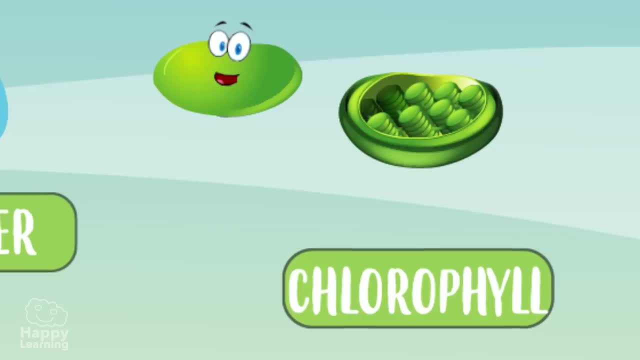 dioxide, obtained from air and water, and chlorophyll, which is a green substance that's also used to make food. Photosynthesis is a process in which plants make their own food. Photosynthesis is a process in which plants make their own food. Photosynthesis is fundamental for performing photosynthesis, since it could not happen without. 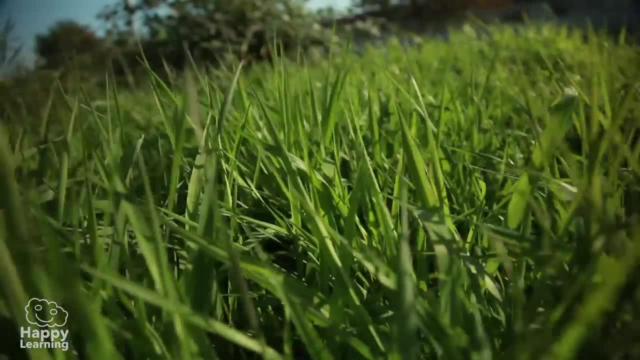 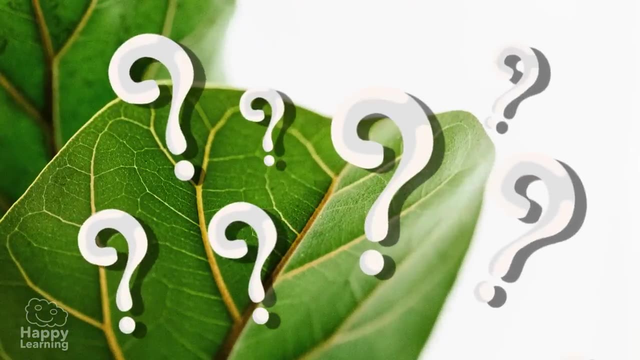 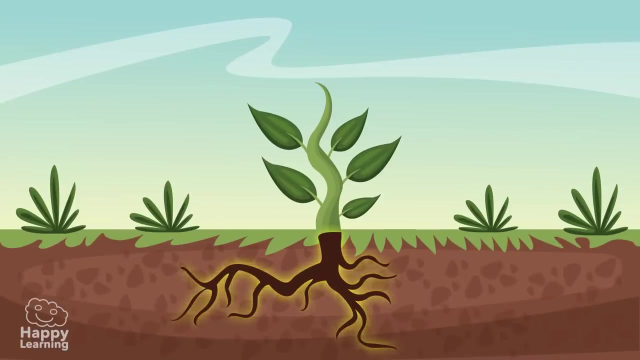 it. By the way, chlorophyll is what gives all plants their green colour. But how does photosynthesis take place? Look at this plant. As you can see. its roots are anchored to the ground and through them the plant absorbs water. Photosynthesis is a process in which plants make their own food. 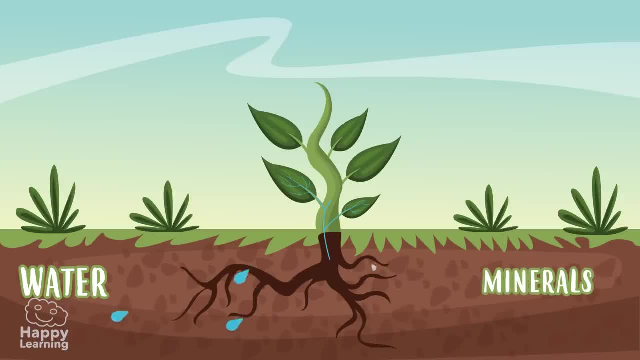 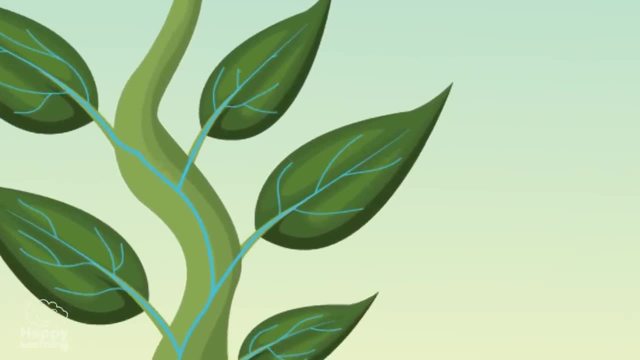 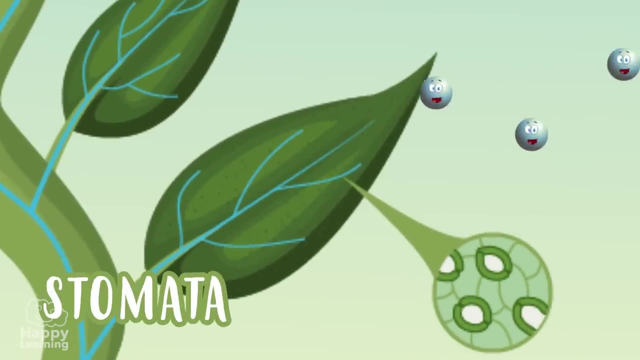 Photosynthesis is a process in which plants make their own food. Photosynthesis is a process in which plants make their own food. The leaves are full of tiny pools called stomata, which absorb carbon dioxide that the air in their surrounding contains. All this, containing water, minerals and carbon dioxide, is called raw sap. 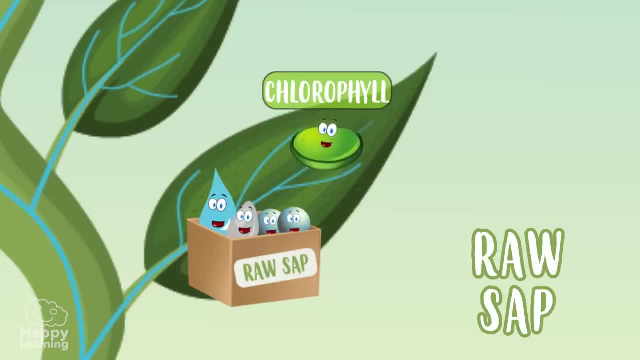 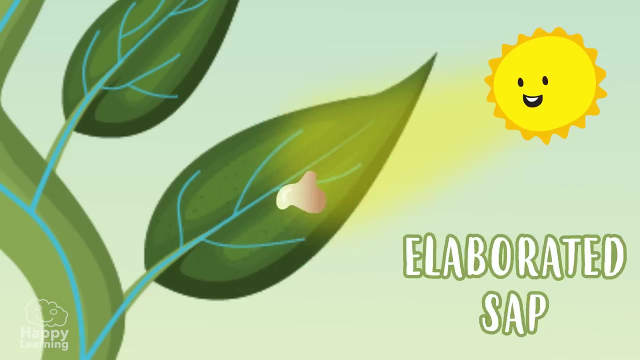 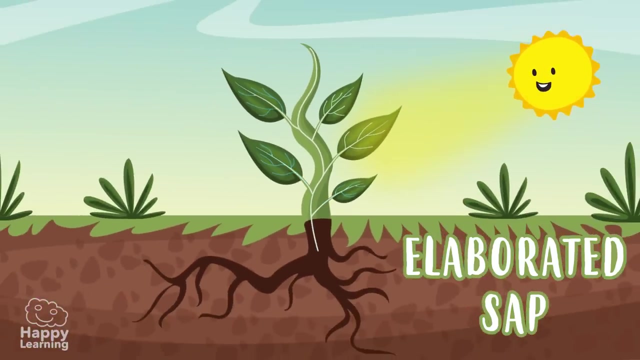 Now it's chlorophyll's turn. The chlorophyll in the leaves has all the necessary ingredients for photosynthesis to take place, And when it receives sunlight, the process begins by transforming the raw sap into elaborated sap, which also circulates around the plant and works as food. 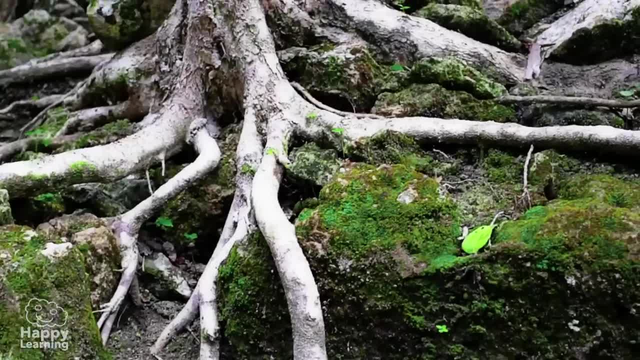 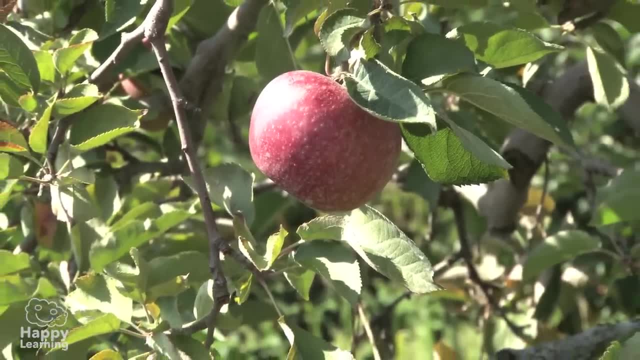 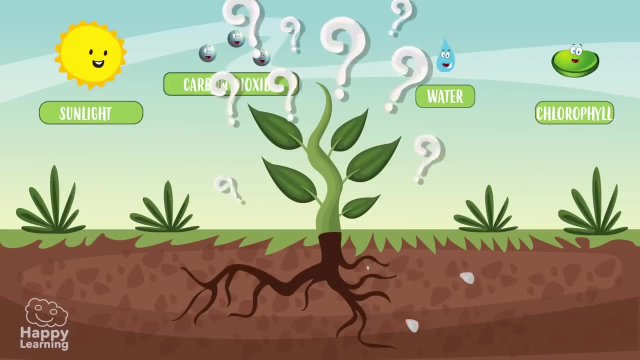 All plants feed from elaborated sap and they store it in their roots, like a carrot, or in their fruit, like an apple or a pear. Now we know how to make chlorophyll, We know how photosynthesis takes place, but why is it so important? 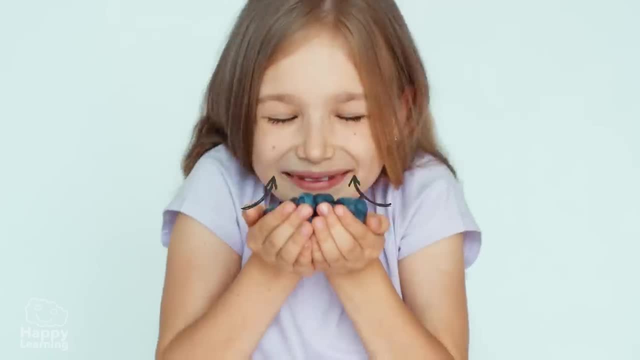 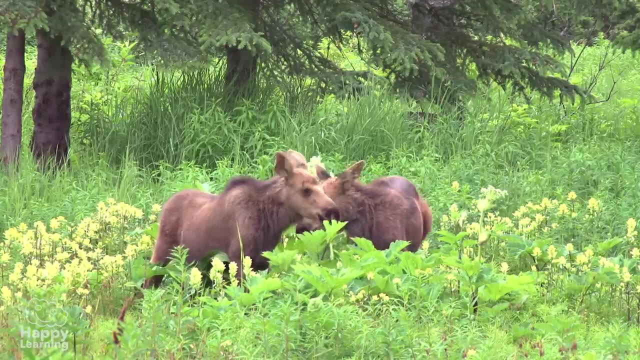 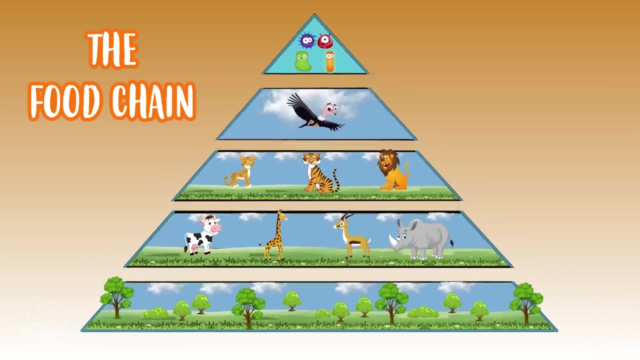 Without plants, there would be no life on earth. We wouldn't have oxygen to breathe or food to feed on. You already know that herbivores eat plants and carnivores eat herbivores. Plants are fundamental for the food chain And they are the most important part of the food chain. 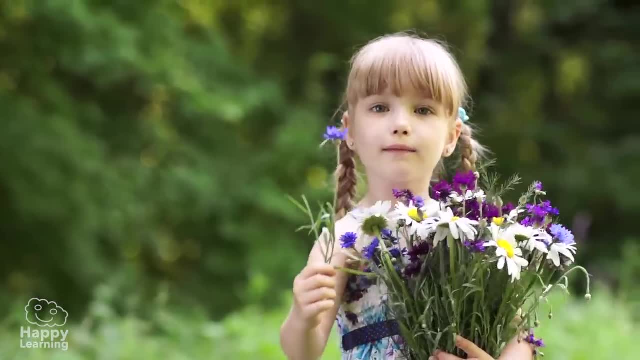 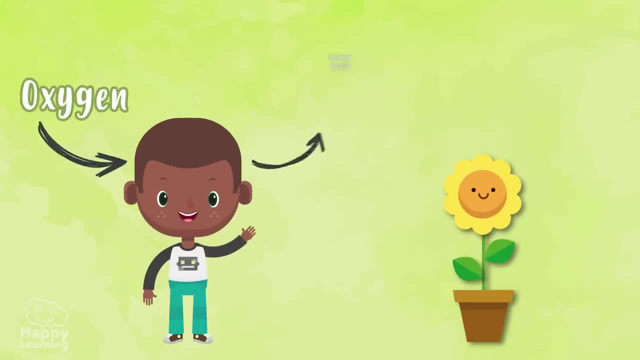 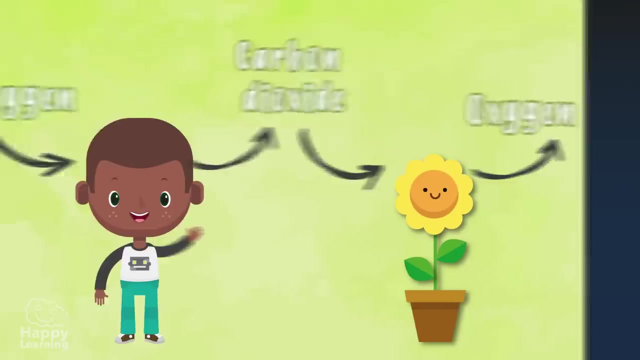 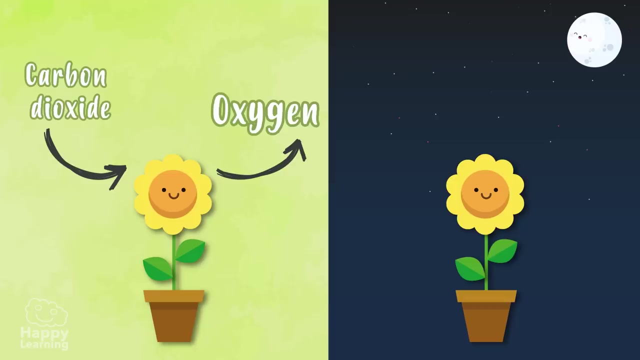 And they are the most important part of the food chain. They are also fundamental for our respiration. Actually, when humans breathe, we turn oxygen into carbon dioxide- Quite the opposite of when plants perform photosynthesis. A curious fact you need to know is that at night, because plants don't have sunlight,